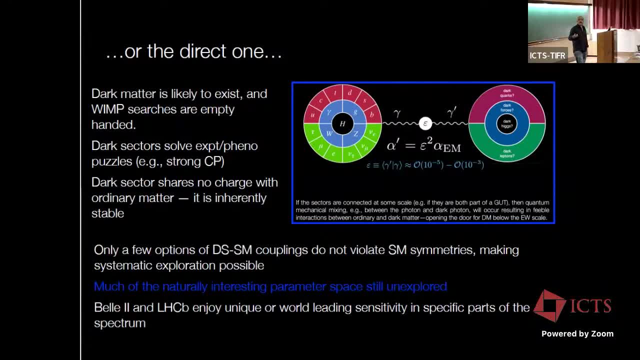 to many, both for dark matter and to many other puzzles, And so there are only a few options of coupling that do not violate standard model symmetries which make the systematic exploration possible, But on the other hand, there are not enough results for making setting very real strong. 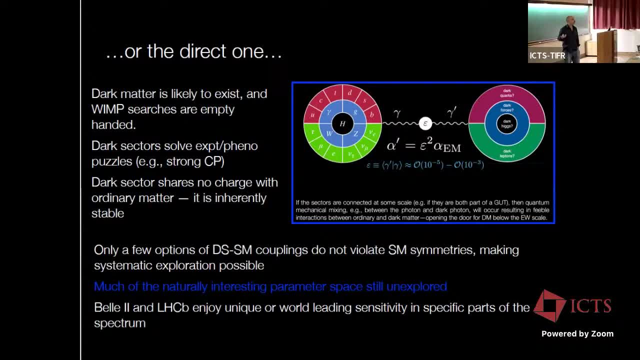 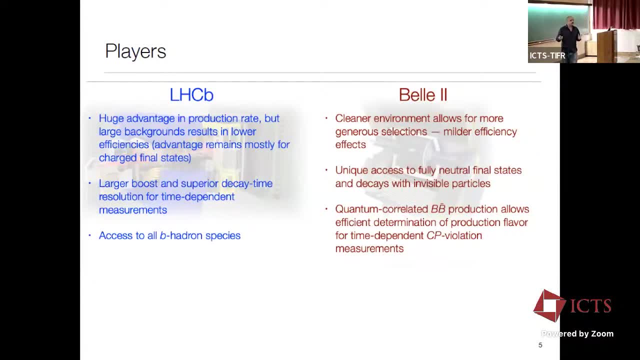 constraints, So we are in a very nice position to investigate those, And I will briefly touch on those two. So these are the two players. In essence, LHCb produces many, many more signal events and much more displaced from the primary vertex, which is an advantage. 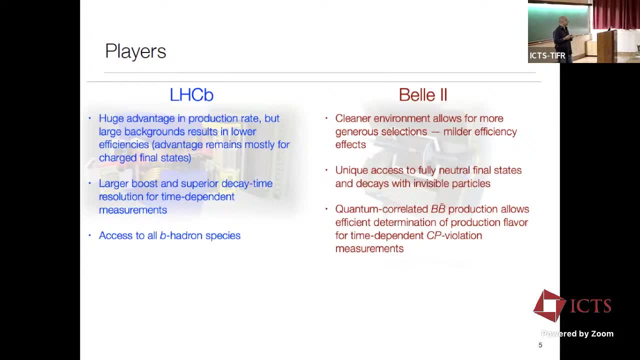 But it's hard to reconstruct final states that contain neutrinos or pi zeros or photons. Well, two produce much less signal In a much clearer environment, with more hermetic detectors, which makes the reconstruction of final states with photons, pi zeros, neutrinos easier. quote unquote. 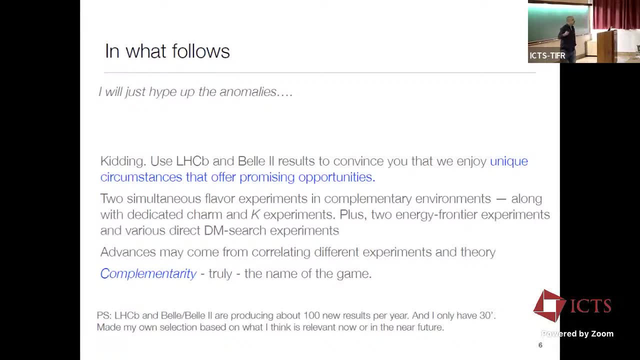 So in what follows I will just hype up the anomalies. Now. it's not true. I will just try to tell you what I just said at the beginning and try to make the case for a unique opportunity in the field of flower physics, but also beyond that, of having a 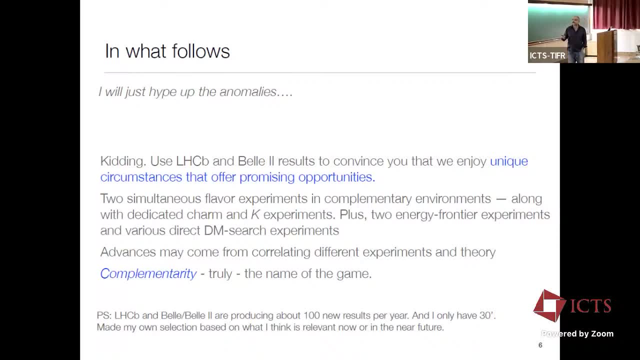 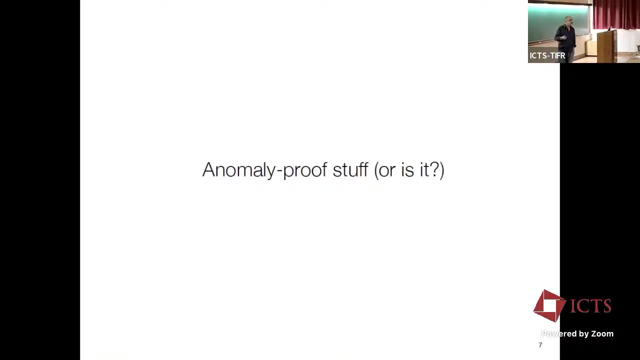 two experiments running simultaneously in complementary environments, And here complementarity really is the name of the game. So since apparently no talk is sexy enough without many mentions of the anomalies, I will try also myself here, And I will start from material that is supposed to not show any anomaly, the stuff that are 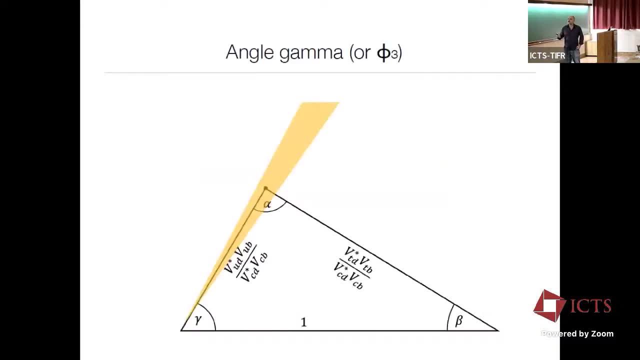 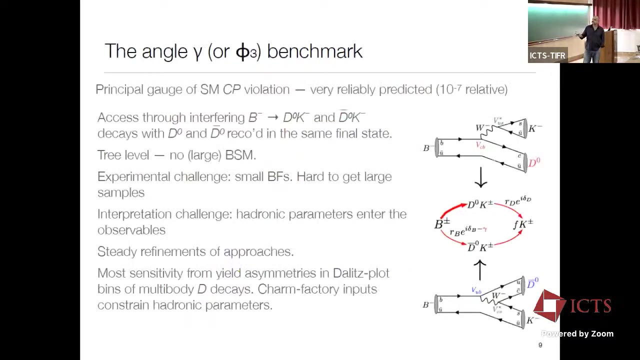 rooted in the three-level standard model And of course, the first is The measurement of the angle gamma, or the VUB phase, roughly speaking. which is this guy here which determines the size of CP violation in the standard model? essentially, 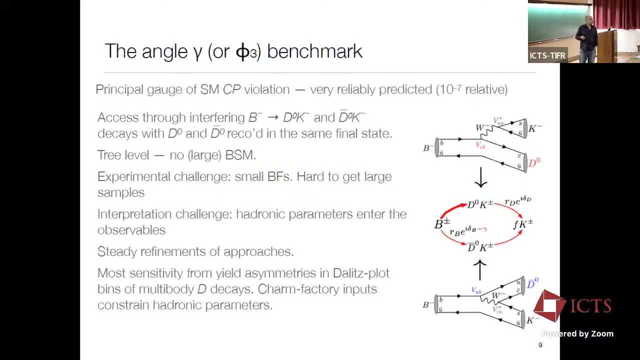 And this is a very nice quantity because if you measure it to 3D case, where you do not expect large new physics, it's actually a very robust gauge of the standard model with a very precise prediction of one part per million or so. 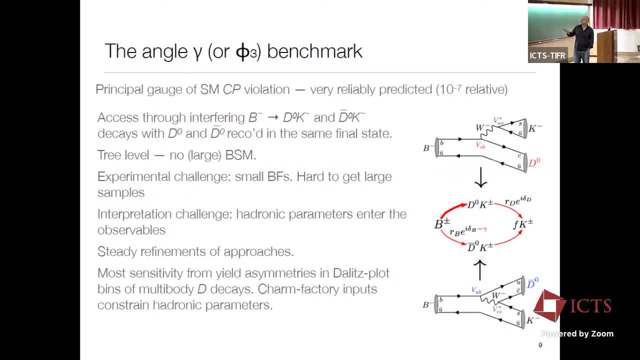 And you actually see this through the interference of these decays of B minus to D0K minus or anti-D0K minus, And you can see that this guy is sensitive to VCB, this one and other, to VUB, And then, of course, you have some hydronic parameters associated with the decay amplitudes. 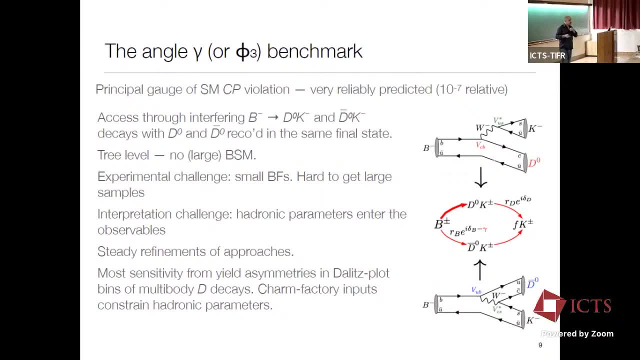 But in the end, the experiments and the theorists have developed a very, very sophisticated and careful way of extracting gamma of phi 3 in a very, very sophisticated way. And this is the first experiment, And this is the second experiment, And this is the third experiment. 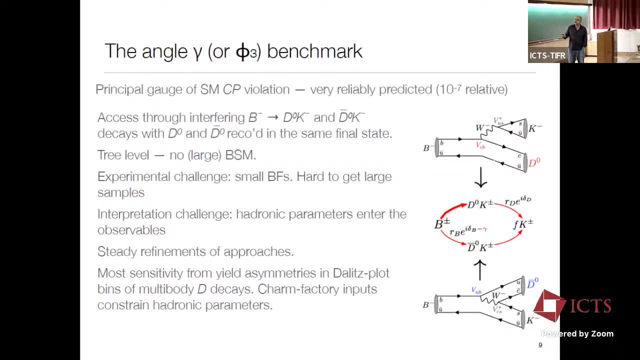 And this is the fourth experiment, And this is the fifth experiment. This was done in a very precise way, from B to D0K, in case And basically the most sensitive method is based on some looking at a C-metrix distributed. 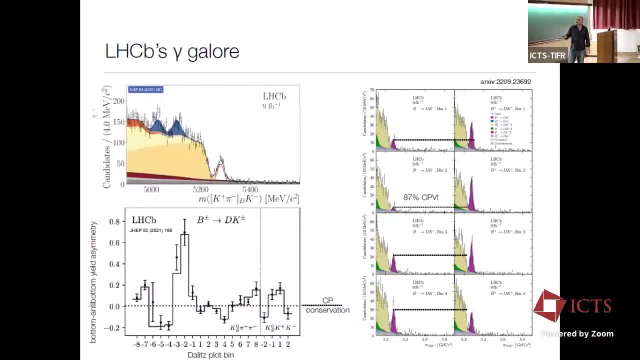 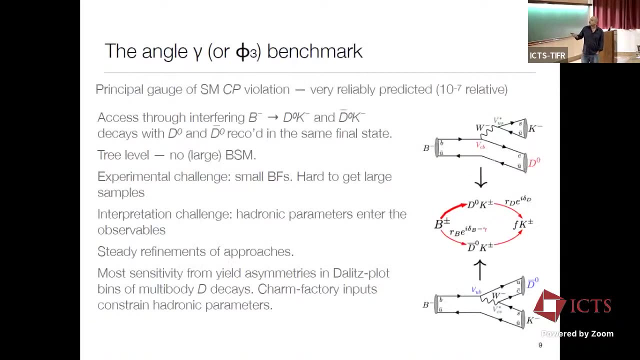 in opportunely chosen bins over the Dallas block. Yeah, You mean new physics in the trees? Yeah, But you would have many signs in many other decades. right, You would have you know deviation in many other decades, Because B2 charm is favored. 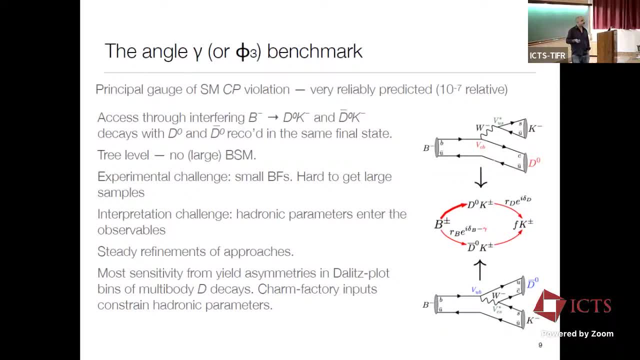 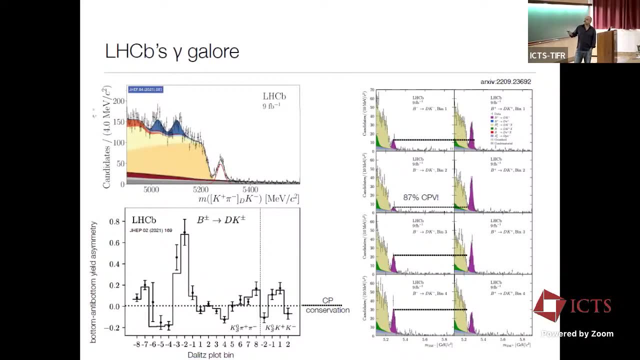 So you would have many other signs of this happening in many other channels. right, And at least if I got your question right, All right, So this is really the terrain of LHCb. that combines many different measurements. I'm not gonna go through details. 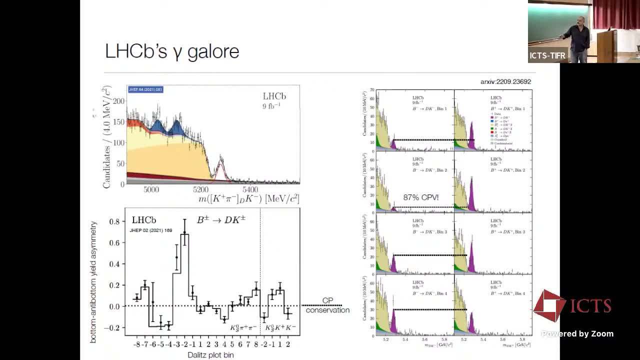 This is the most sensitive one. So you see, these are the what, the asymmetry that you observe as a function of some beans in the Dalitz plot, And you see that if there was no CP violation, you would expect all the things scattering around here. 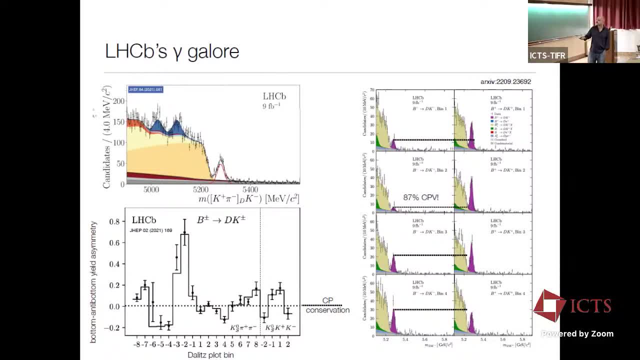 And you can clearly see that there is large CP violation, very precisely measured. A more perhaps intuitive way of seeing it is another channel for a decay of the charm in four atoms where you can see that in some beans you have even 90%, almost CP violation. 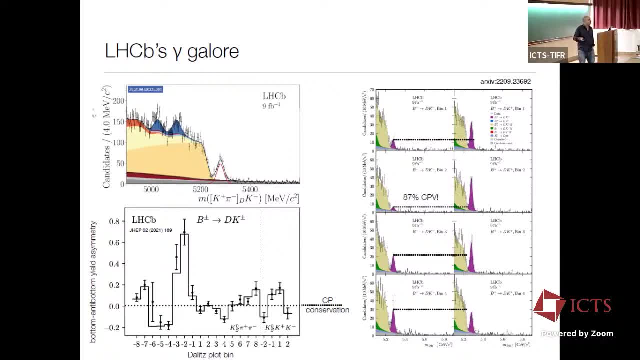 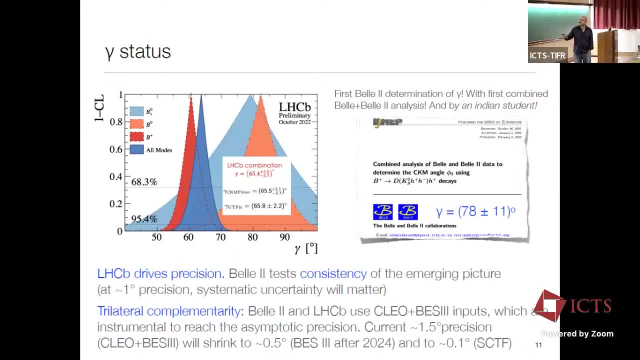 You see, the difference between these two purple peaks is huge. okay, So LHCb does this measurement and combine them together. We find the determination of the gamma with an error that is less than four degrees. Okay, Less than four degrees. Bell two here cannot compete on the precision. 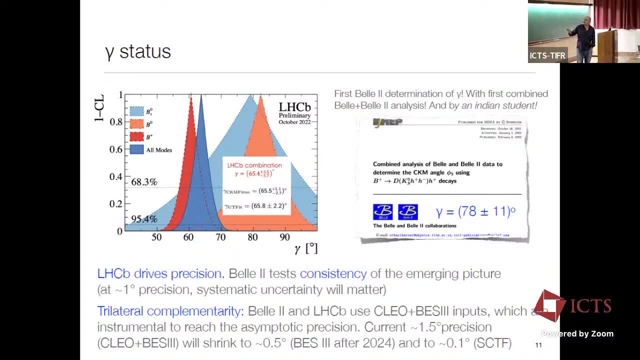 even though bell two has the first result, with a combined bell and bell two analysis in fact, And it's nice that it was actually driven by an Indian student. And of course you can see from the uncertainty that we are not competitive with LHCb at this time. 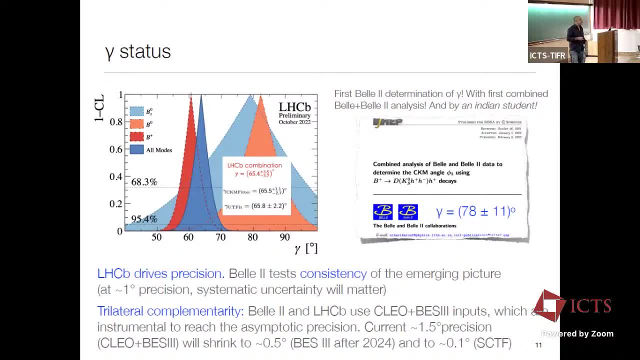 And of course you can see from the uncertainty that we are not competitive with LHCb at this time. And of course you can see from the uncertainty, But down the line, when the global uncertainty will be of the order of one degree or less, we expect the systematics will be important. 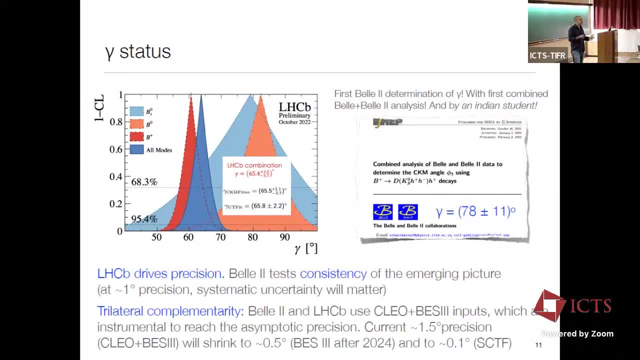 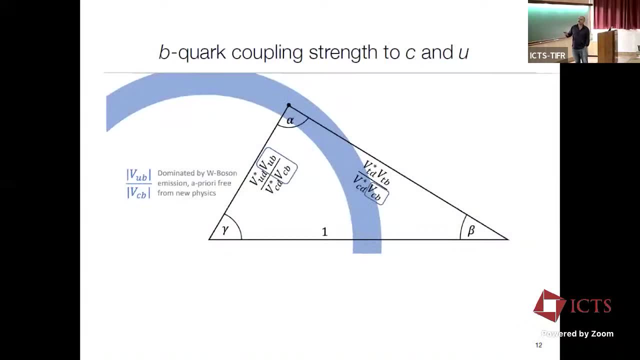 And at that point it would be very important to have two different experiments with different systematics checking each other. Then- another thing that is dominated by 3D case- are the measurement of the strength of the B-quad coupling to C and U. 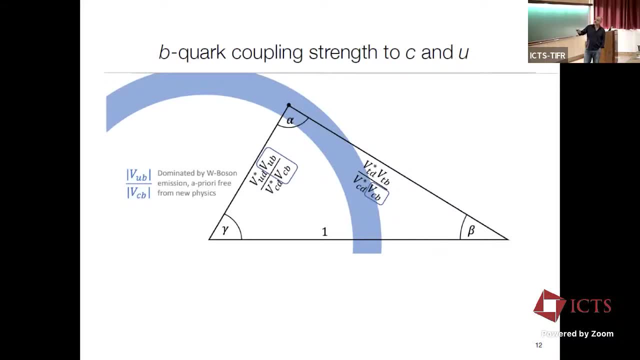 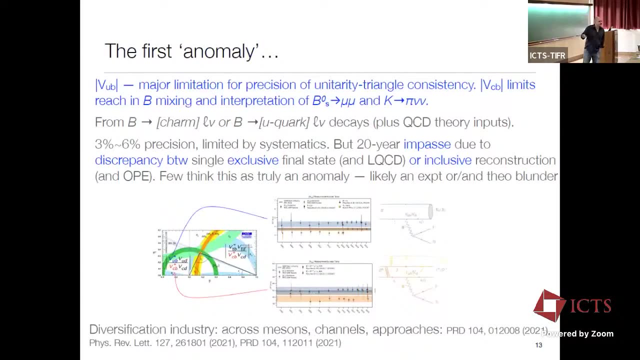 These are the guys that determine these apex, here, through this constraint, And here, in fact, there is the first anomaly, if you want to call it such, is the fact that the determination of these parameters happens through semi-leptonic decays. 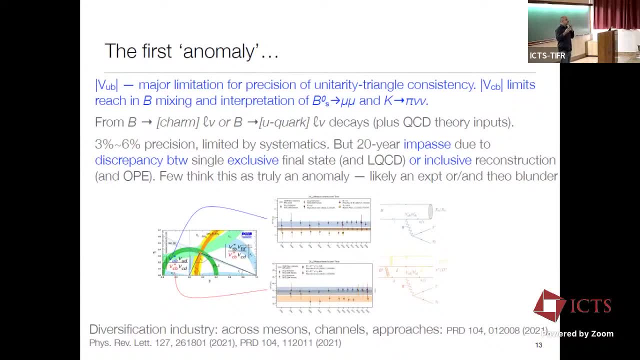 And you can choose to reconstruct only one channel, one semi-leptonic channel, then combine with QCD lattice inputs and get one determination, Or you can have additional, So you have a different determination where you actually look inclusively at many final states. 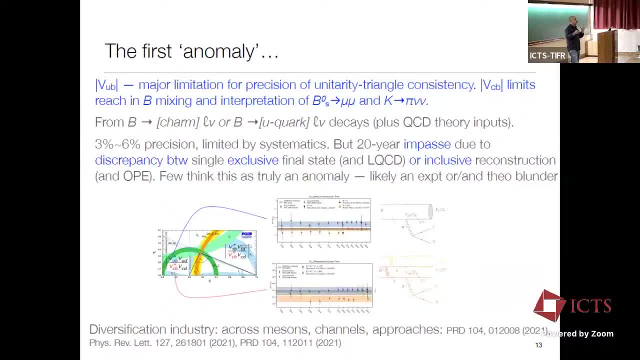 And you use operator product expansion, QCD and you get another determination. But you expect these two guys to converge to the same value And you can see from these bands here that there is both in VUB and both in VCB and in VCB a difference, a systematic difference between the inclusive and the exclusive determination. 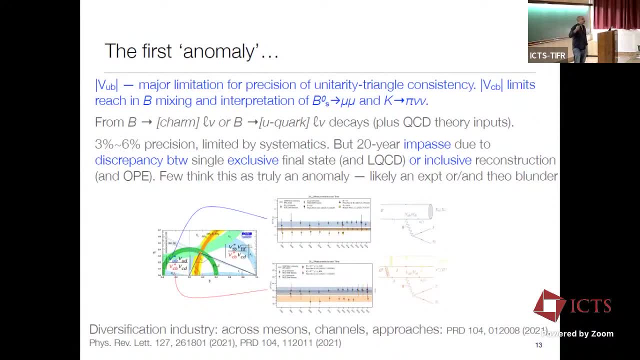 So many call it an anomaly. Some people even try to interpret it in terms of new physics, But I think that most people think this is likely to be either a theoretical or an experimental blunder, most likely associated to the inclusive part, which is the most difficult. 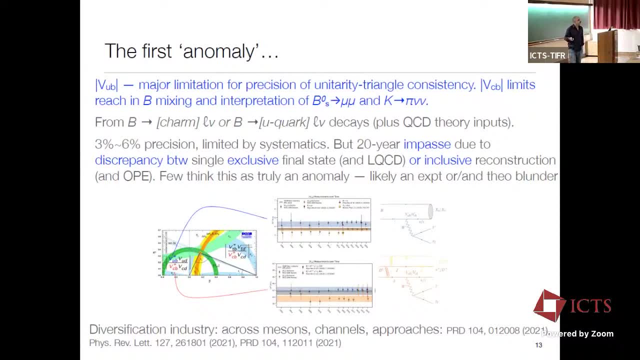 And so here, what we're trying to do is to diversify the portfolio. You know, when the market is uncertain, you diversify, And so there are many measurements across many mesons, channels, approaches, and here is a short list. 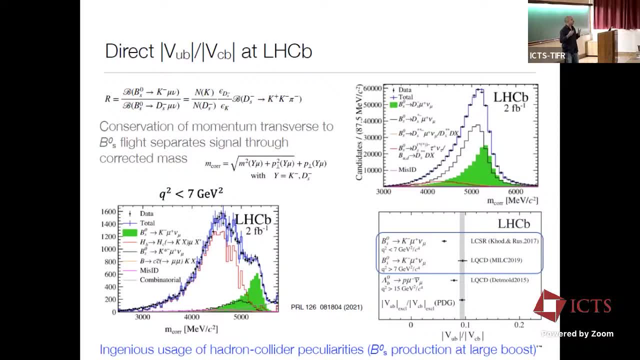 And the nice thing Is that, while this has been traditionally the realm of B factory experiments, LHB has been weighted, weighting very, very strongly, with a very nice measurement directly of the ratio, which is the important quantity, between VUB and VCB, through this ratio of branching fraction of BSDKs. 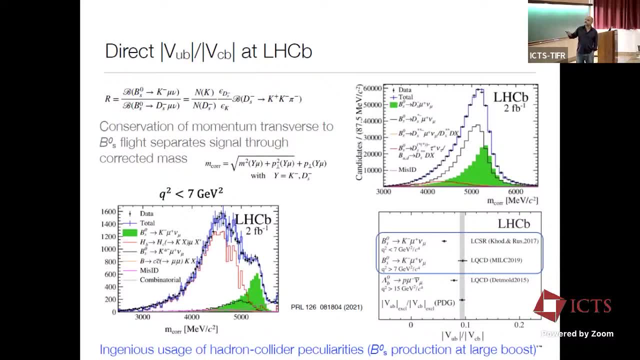 So you have BS to K mu nu, which gives you the VUB thing, and BS to DS mu nu, which gives you the VCB, And then, of course, these are very difficult analysis Because you have neutrinos in the final state and you don't have discrimination of the signal. that is very precise. 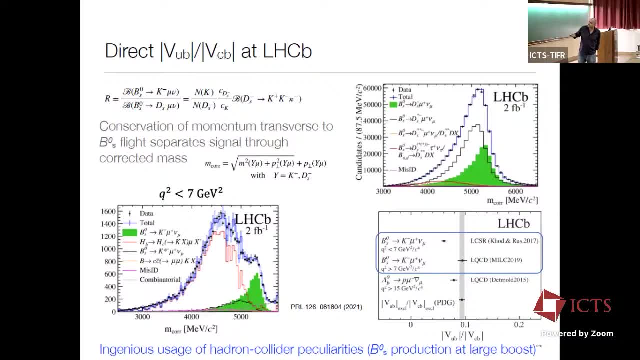 You have to. you know, see the signal is this green thing? You have to try to fit your signal, which is barred, in this large background. So the sample composition is very critical And you have to do many, cross-check, many you know control channels to make sure you understand what you're doing. 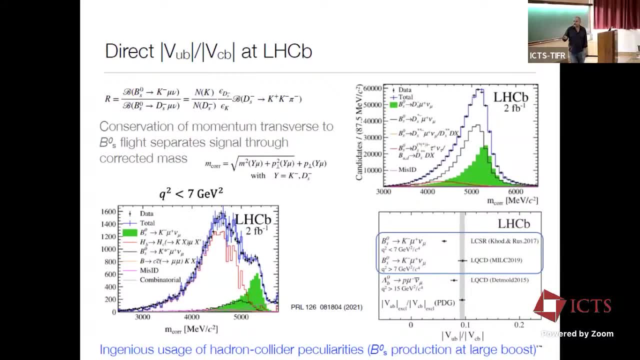 And in the end the results are very, very precise, And I think this is a very Nice demonstration of an ingenious use you can do of the peculiarities of hydrogen collider physics. So you have B sub SDKs which you do not have in, at least you do not have in large abundance B factories. 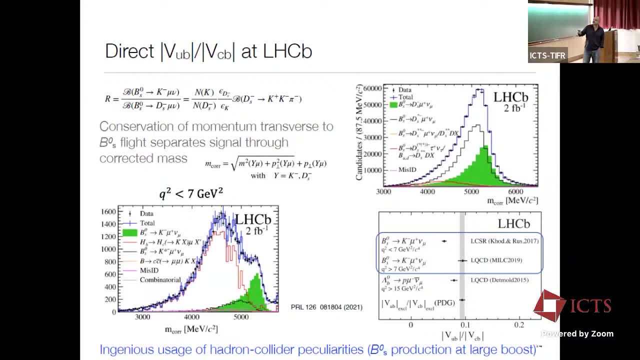 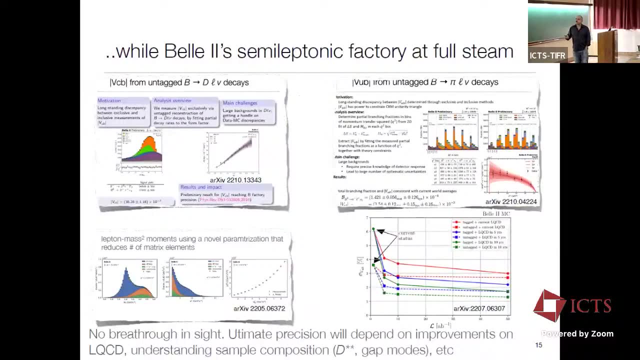 And you have large boosts which gives you the possibility to construct the BS direction and build these variables here. Bell 2 is too early to provide actually very competitive results. But the factories, You know we are in the very first stage Of the whole system with many different results on view B and VCB in various different ways. 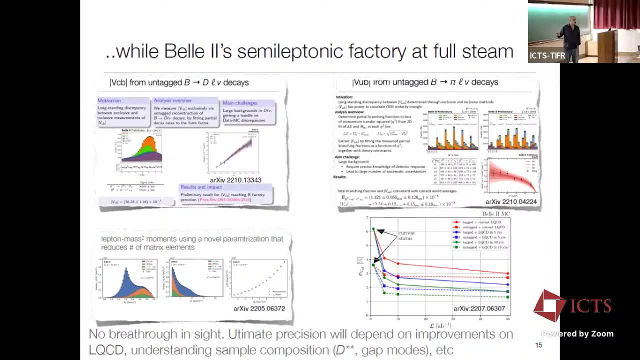 So, if you look at the future, we're looking at something that, depending also on lattice QCD advances, we go to precision of the order of 2% or so, But of course we will only get there if we figure out the discrepancy between inclusive and exclusive, which is probably the most pressing issue here. 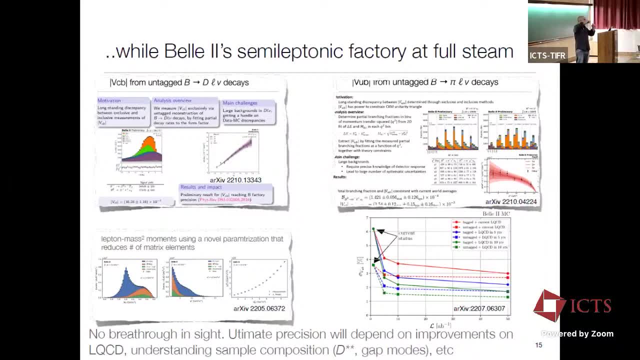 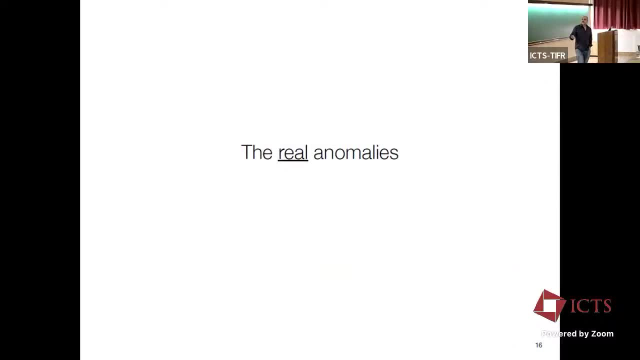 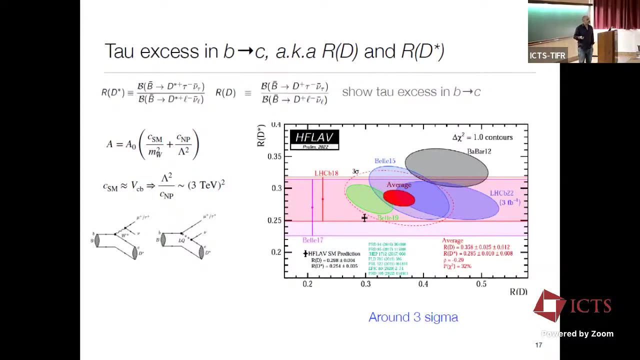 Because without that we will just make the discrepancy a larger, with more precise measurements. Now let's go to the real anomalies. Let's start from the tau excess that has been observed by various experiments since already five or seven years in B to C transitions. 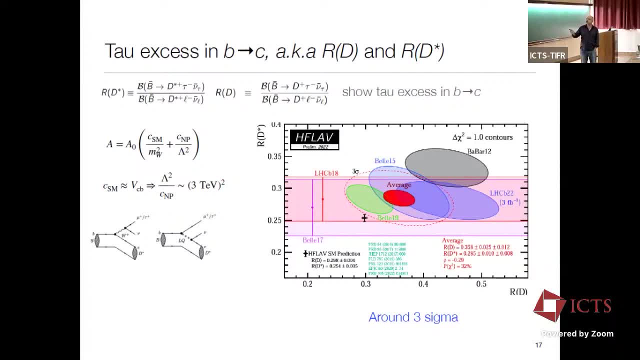 Again here. this is three transition. This is also called RD and RD star And basically you measure this by measuring this ratio of branching fraction between D star to tau nu and D to tau nu versus the lighter leptons, E and nu. on the denominator. 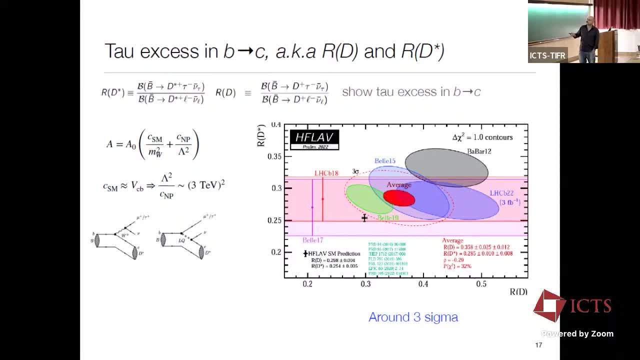 And what you see here is that the standard model prediction is somewhat far from the average of the other experiment. Three sigma: 3.2. sigma 2.9 is not important. There is a pattern that is consistent of being far from the standard model prediction. 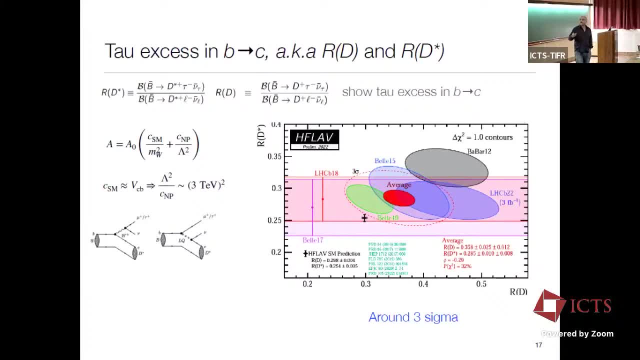 So, if you want to, if you want to interpret this in terms of sorry, ineffective field theory, you can imagine that there is some, you know, for natural coupling, some standard model, non-standard model, physics of the order of a few GV mass. 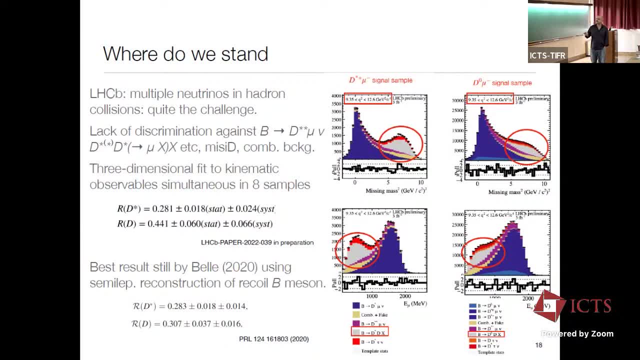 Where do we stand here? This is a longstanding discrepancy, So we have been continuing to investigating. Last, one of the last contribution has been the simultaneous measurement, the first simultaneous measurement of both R D star and R D by LCB in Hadron- collisions. 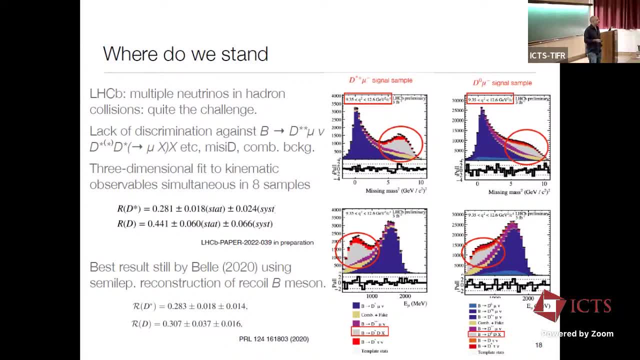 I think this is one of the most difficult measurement one can try to do in Hadron collisions because the numerator has three neutrinos. So it's really very, very difficult to find a distribution where you can distinguish the signal. You see, this is the data you see. 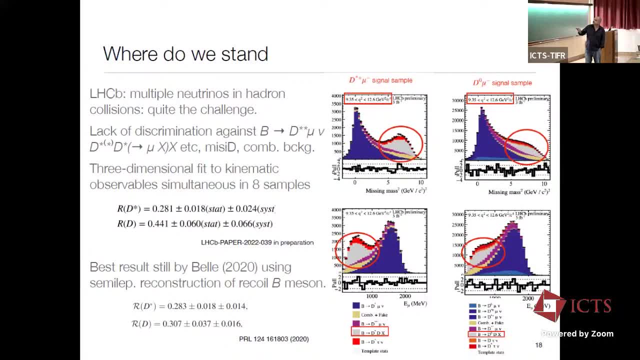 and this is what you're trying to separate, to separate using simultaneous feeds of signal-enriched samples, control channels, et cetera, et cetera, et cetera. This looks very, very difficult And it is. these are very long analysis. 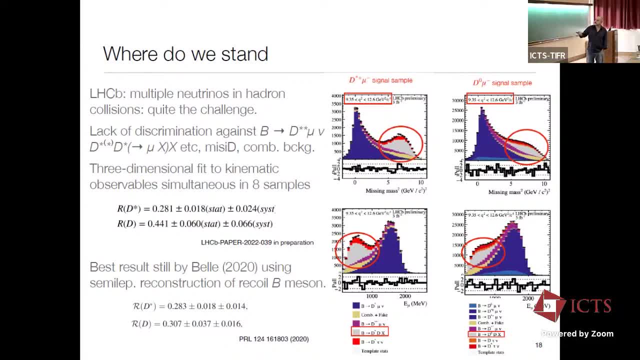 but in the end the results are very nice And they're not as precise as the best results from the B factories, but we are getting there. We are getting there. So this is just an example of what you can really do when you have so much signal as LCB has. 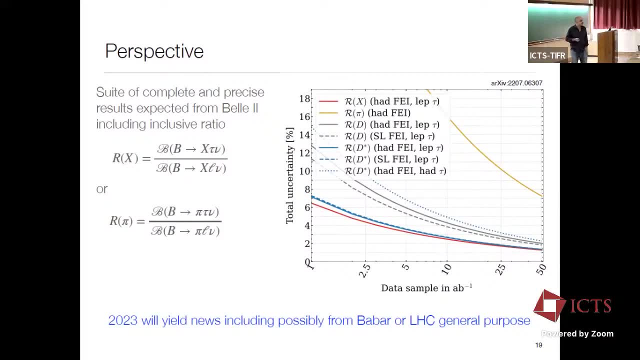 So where is the perspective here? I think that you know, despite the LCB efforts, I think here the drive will be on Bell two, because Bell two these analysis are significantly easier in B factories and Bell two can also access other quantities. 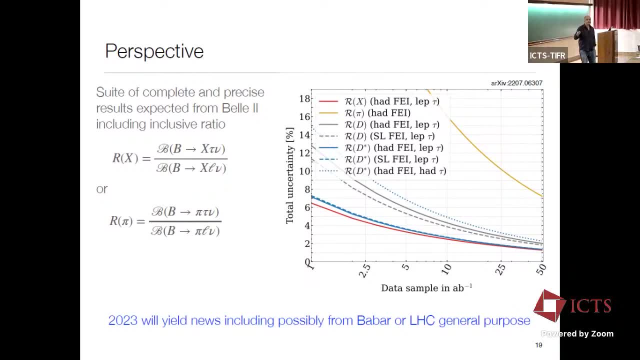 not only R D and R D star, which is the exclusive quantity, but we can also measure R X. So you will just not reconstruct the Charm meson and you just you can look at it inclusively, or you can even do these ratios using pions. 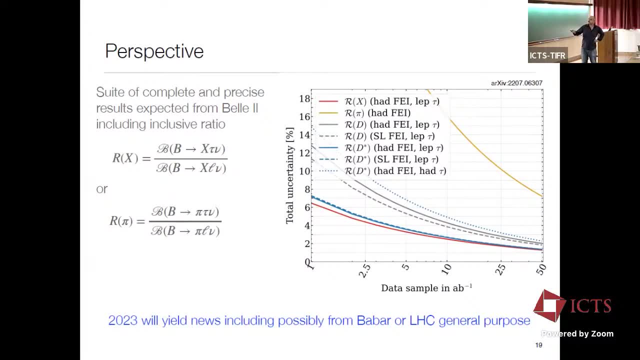 So this is a plot that shows, as a function of the data sample sites, where the procedures of these various ways of accessing the same anomaly can get us, And what I think will happen next year is that we might have new results not only from Bell two, but also from Bell. 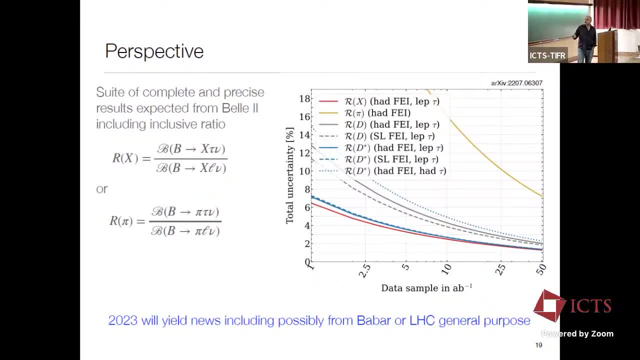 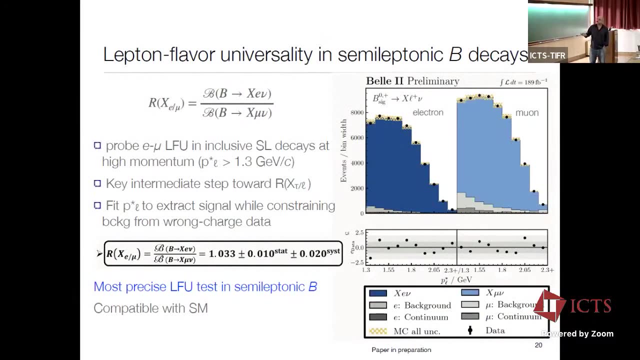 and maybe also from CMS, Atlas, et cetera, et cetera. So I think this is one of the things in which we want to focus our attention soon, Part of this process of looking at the inclusive ratio, something that is basically has been done only. 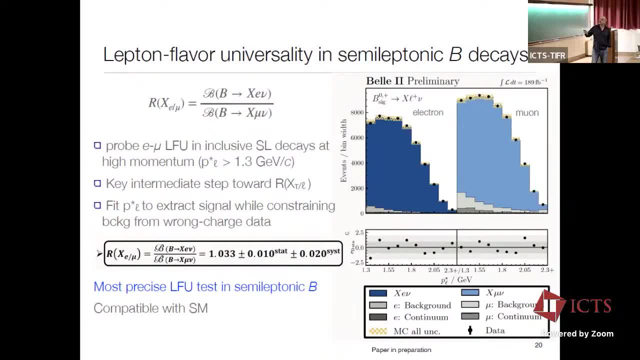 in the early 2000s at lab and never done after, is to look at the ratio of the electron over muon, which is one of the latest results from Bell two, where you basically try to find lepton flavor universality between the two light leptons and you do it in a high 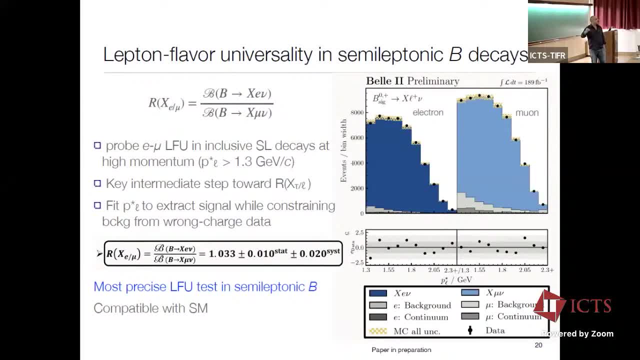 part of the lepton spectrum when you do not have no more any. that taos and the results are actually very, very intriguing. We have, of course, we have a result that is compatible with the lepton flavor universality. it's one. 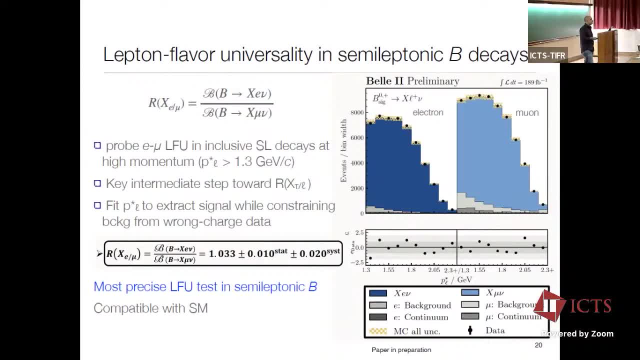 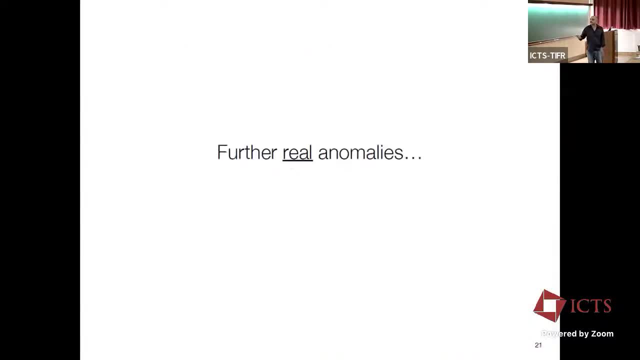 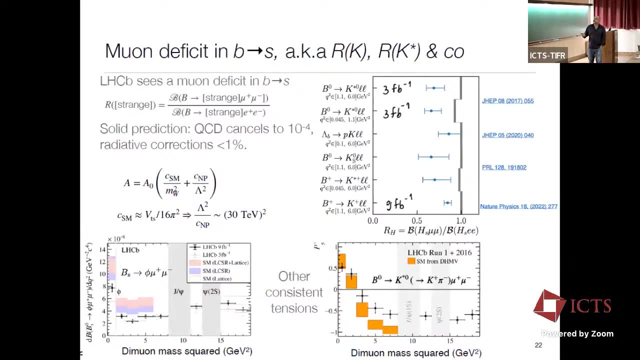 but the uncertainties are very, very competitive And this is was something that Bell two did not expect was just an intermediate step in the analysis of the rx, of the inclusive one, For the real anomalies are those seen basically by, by LHCb only in mu, on deficit, on B2S transition. 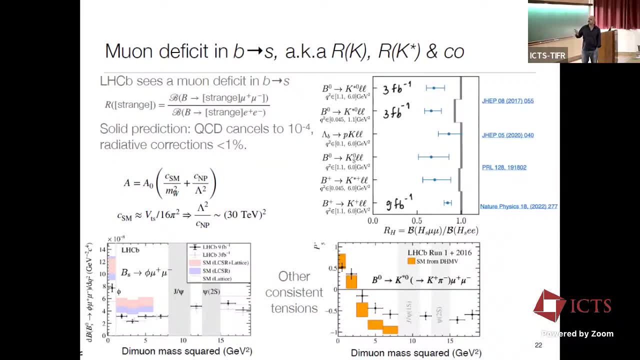 which are also called Rk, Rk star, Rk short, et cetera, et cetera. But basically also here you're just looking at the ratio of two rates of B2 strange mu mu over B2 strange EE. 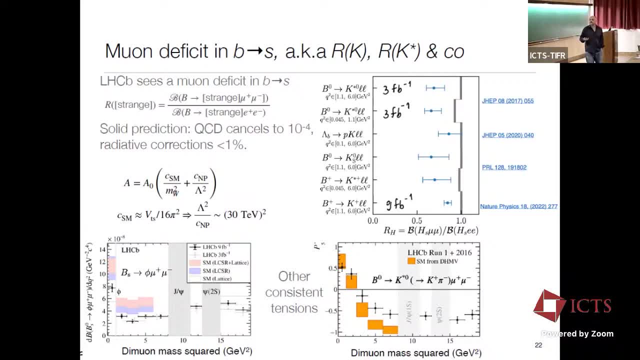 These things are a very solid prediction, as QCD uncertainties are very small and radiative correction are also small, And you can see here in this collection of results that the measured values are all lower than what you would expect from lepton flavor universal, So from the property that leptons only differ by themselves. 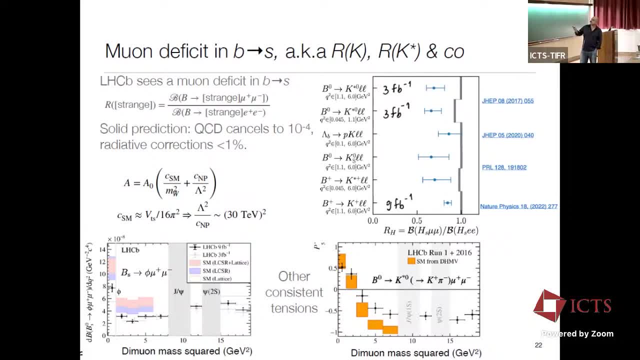 only by mass, nothing else. And this coherent deficit is what excited many people in our field. Also, because it's a very it was accompanied by other tensions that were consistent with that. This is a tension in the branching fraction, as a function that the mu mass square. 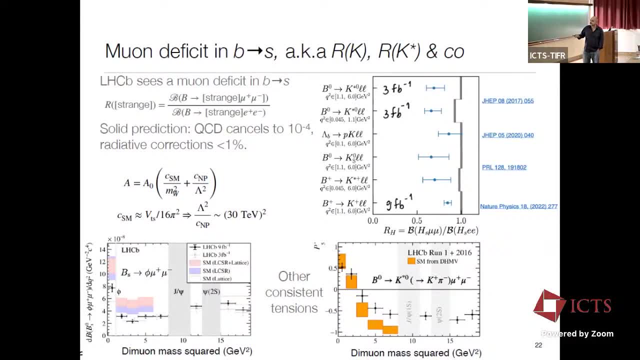 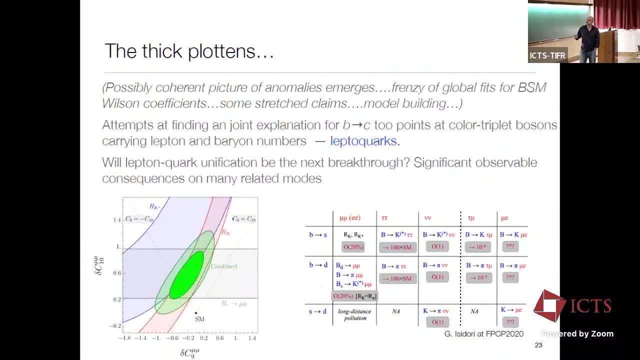 However, here the predictions are more uncertain. This is a tension on a special angular variable that suppress the adrenic unknowns, et cetera, et cetera. So this coherent picture of anomalies have of course triggered a lot of excitation in the field. 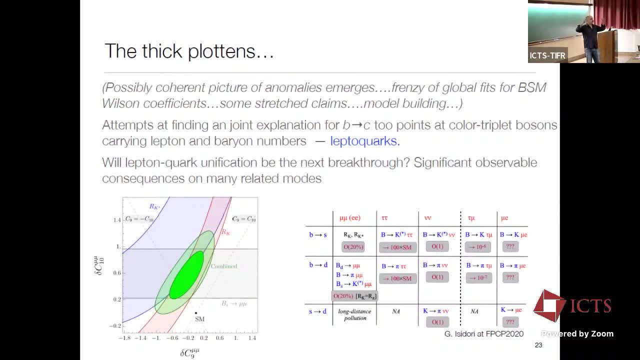 Many people are trying to, you know, fit a non-standard model with some coefficient that were compatible with all of these anomalies. There've been some model building And one of the most popular explanation for this is a revival of the laptop works, which are color triplet bosons carrying lepton. 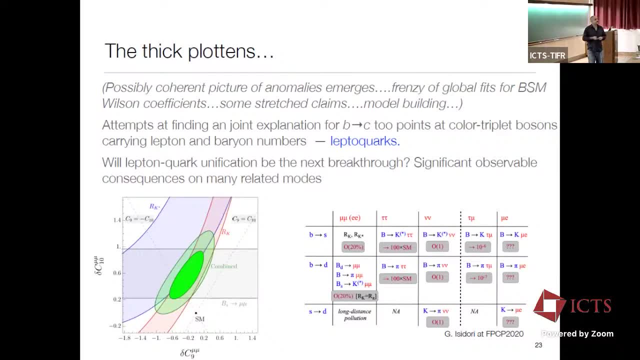 and by the numbers would suggest, you know, a next unification between lepton and quarks. And you can see the interesting part here is that some of these model predict or suggest significant enhancements or changes with respect to the standard model prediction in many other families of channels. 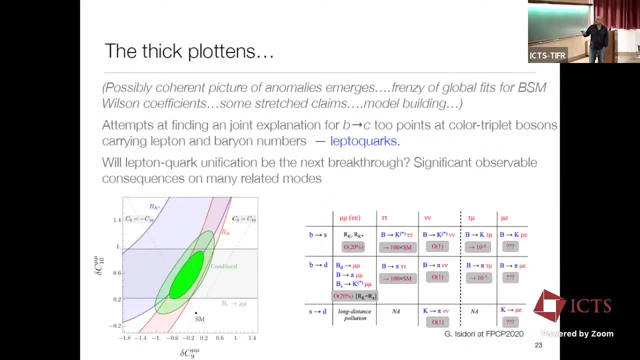 So K star K tau tau, K star nu nu K tau mu, et cetera. So it's obvious that from an experimentalist point of view, the next thing to go is to go and look at those guys. But before getting too excited, let's also examine. you know. 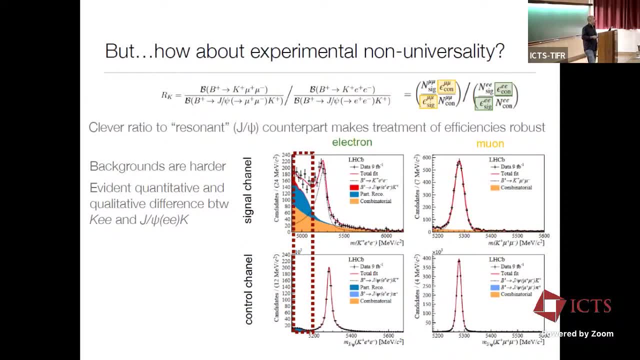 the other things that we can look at. But before getting too excited, let's also examine the possibility of experimental non-universality, right? Because while the theory here is clean, the experiment is much less cleaner, especially in hadron collision. 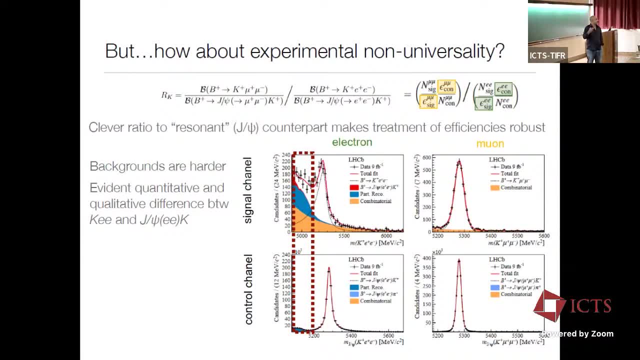 You have differences in efficiencies in reconstructing nuance and electrons And those are nicely suppressed by doing double ratios with respect to the J side, to the resonant channels, okay, So that part I think is very solid. But there are also differences in background. 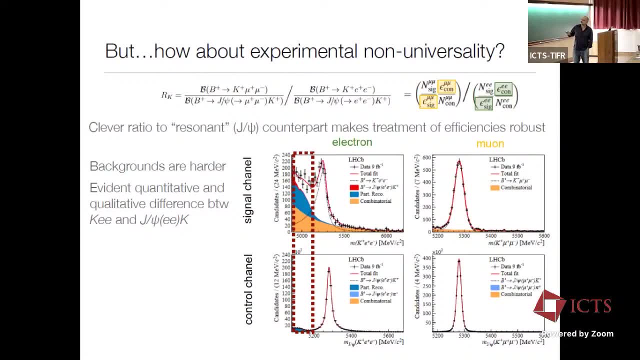 If you compare the background, you get into the electron here. with respect to the background, you get to nuance. you see that there is a lot of difference And this difference is not obviously taken care of by using the normalization with the J side channel. 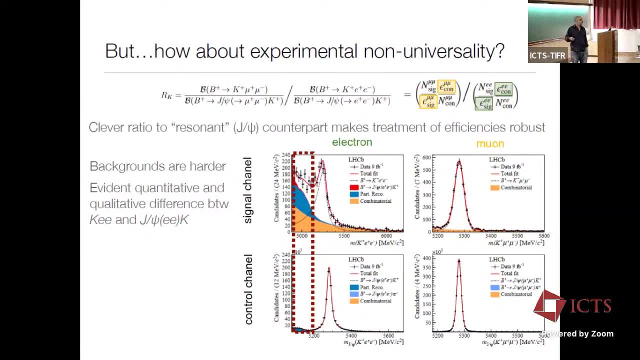 In fact, here this background is in size and in composition quite different from this one. So this is clearly one, two, three, four, five, six, seven and eight. This is one of the delicate points of those analysis. 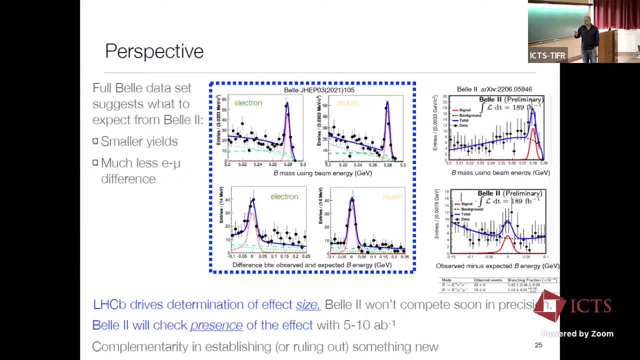 especially in hadron collisions, Because at the B factories you see that the situation is also visually seems more, seems easier, seems more symmetric. right, These are the electrons, these are the nuance. this is a latest Bell result, This is the preliminary Bell two result. but look at here: 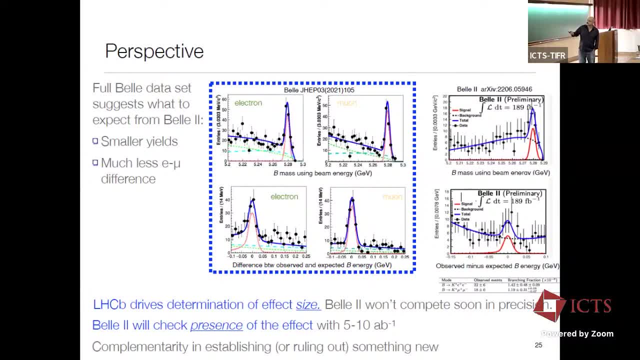 and you can see that the picture of backgrounds, and in both the resonant and the non-resonant channel are much more comparable, in a way. So I think that, however, here you pay, that you have less signal, of course. 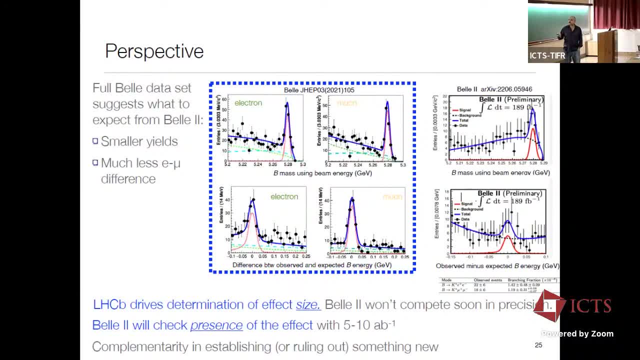 So I think that a nice way of putting that is that LHCb will unquestionably drive the determination of the size of the effect, if there will be an effect, But of course, and Bell two will not compete in the precision, but of course, these considerations about 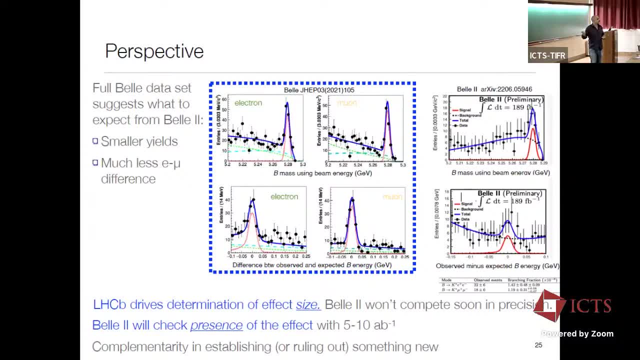 the real differences between electron and nuance, for instance, in the background, will need Bell two also because Bell two, with more statistics than now with five to 10 inverse Atoban, may prove the or the check at least the presence of the effect. 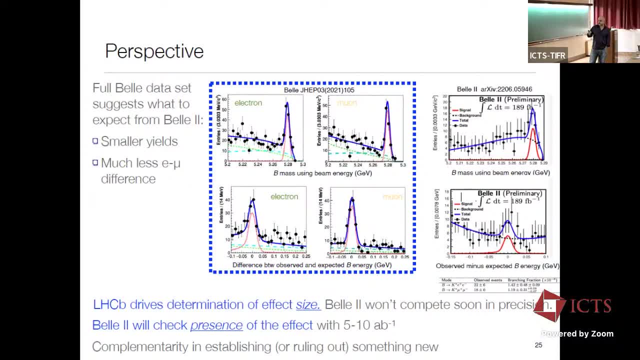 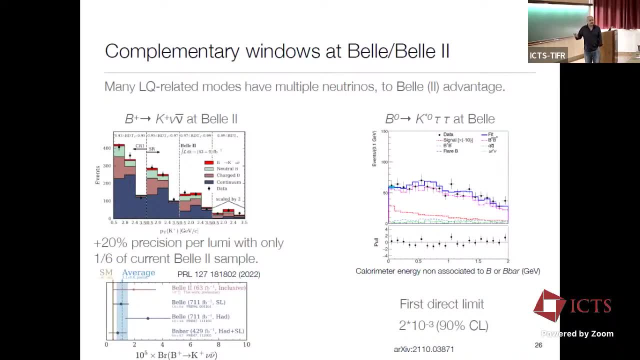 even if not contributing much to the precision. So again, this is a clear case of complimentary Yeah. And of course, another thing is to look at the other channels that are enhanced in the models put forward to explain those anomalies. For instance, Bell two and Bell are doing 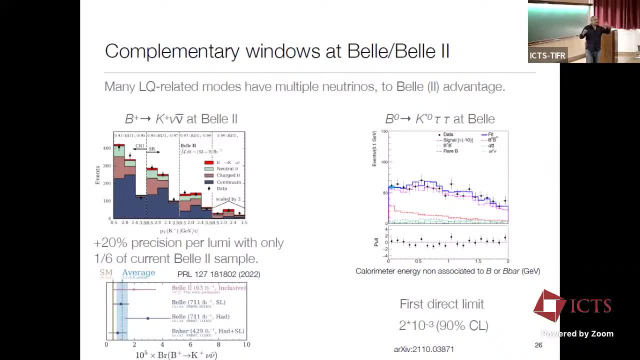 a significant campaign to explore auxiliary channels that expect enhancement if these things like laptop work of non-standard model with super efficient are there. So we have measurement of B plus to K plus Nunu at Bell, which achieves a much better precision with only one sixth. 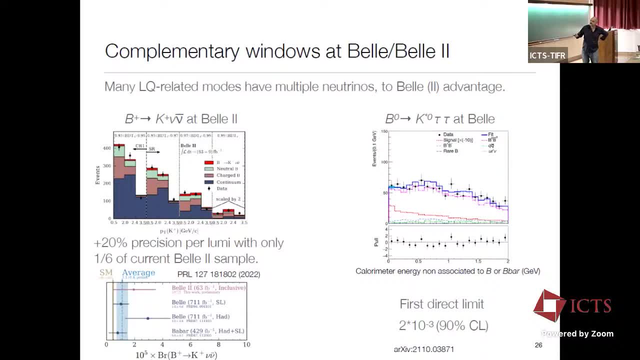 of the current Bell sample. you see we have a precision that is already compatible with the best measurement from the previous B factors with full sample And also we have a recent result of B zero to K- start out our Bell- which it's a very difficult to now. 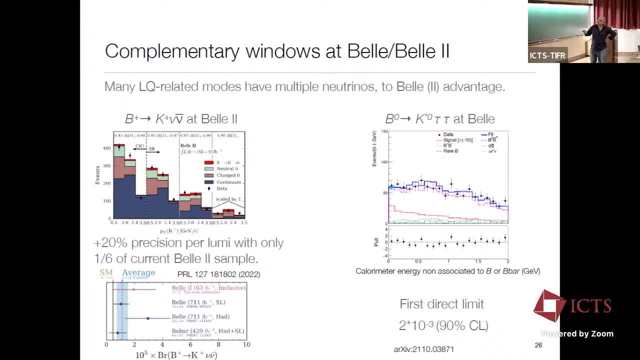 is very, very difficult to see. They look at the signal as a enhancement at zero of the calorimeter energy not associated to a BB bar And they put the first direct limit, that two times 10, to the minus three. So there is a whole campaign going on here. 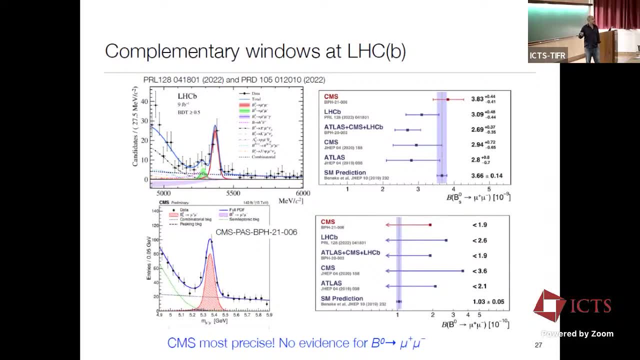 And of course it touches also another very important channel that has been pursued at LHC, especially LHC-B but also CMS, which is B S to Nunu and B to Nunu, with very nice new results, very strong Mediterranean combination, And it's actually very surprising that currently 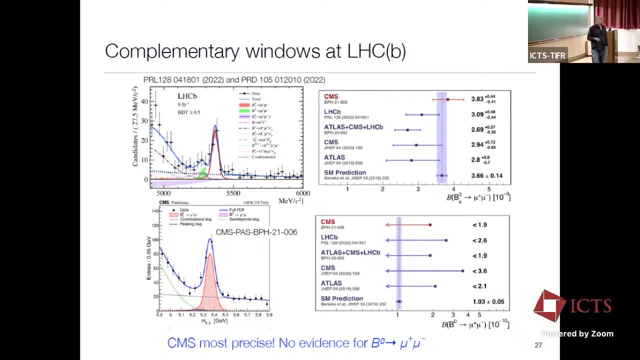 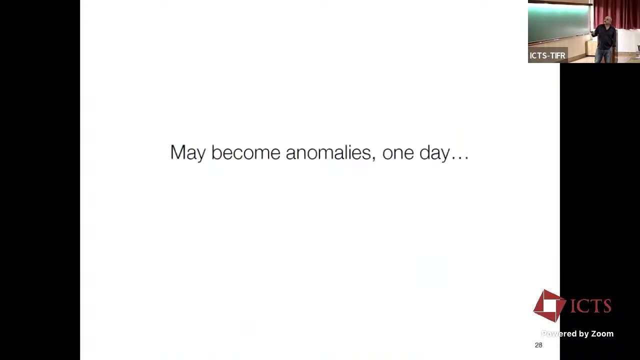 the most precise result, even by a very little, is by CMS. This is really a nice proof of the power of Hadron collision, also in doing precise flavor physics. I'm finishing Some things that are not anomalies today but may become anomalies one day. 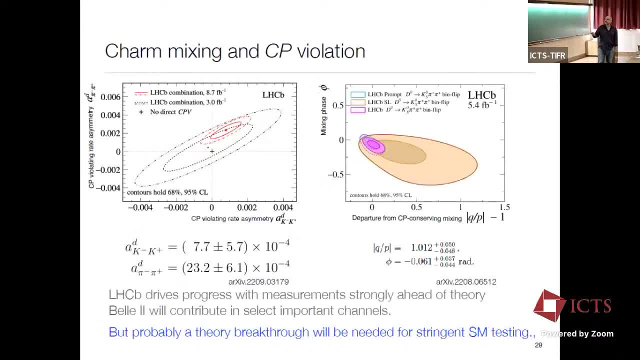 This is just a joke, just to hype up the anomalies thing LHCb is doing a lot in charm physics. order of magnitude advances in our understanding of charm CP violation with the first evidence of CP violation in a single mode here in direct CP violation in pi pi. 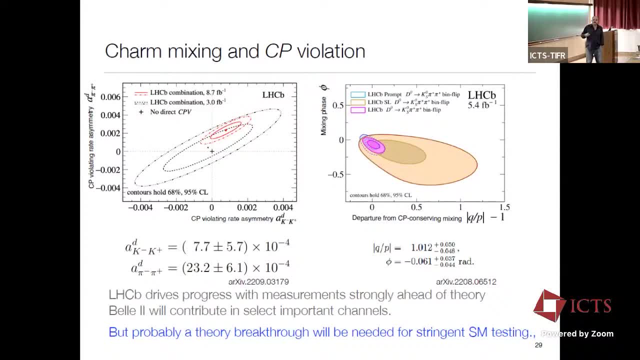 represented in these two plots here, And also the first evidence of a mass difference between the charm eigenstate and the first very tight constraint of CP violation in the mixing. And of course here these things will further improve with more and more statistics. 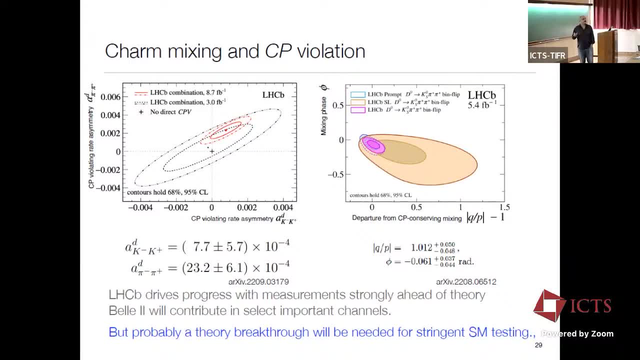 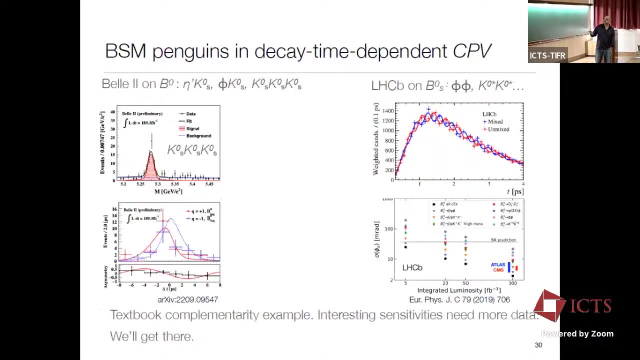 But I think that in order to see whether this stuff is compatible or not with a standard model, we need to wait theory, Because at least my understanding is that theory is currently a bit behind on this for the obvious difficulties associated with charm, mass values, et cetera. 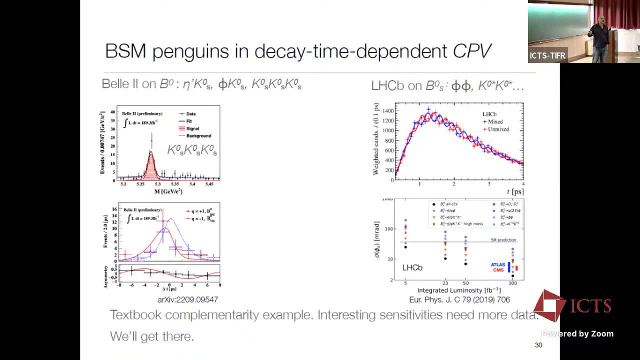 And of course in the meantime Bell 2 will explore and LHCb will explore also beyond the standard model, physics in penguins Through time-dependent CP violation. penguin loops: k-short, k-short, k-short, eta-prime, k-short, phi, k-short. 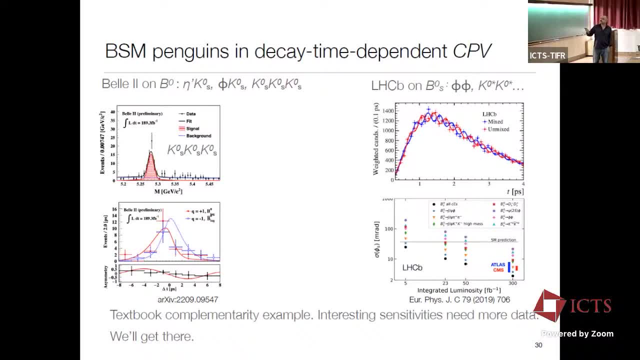 et cetera, et cetera, And the same thing will happen with the b-sub-s phi phi, k-star, k-star at LHCb. So here this is another very clear-cut example of complementarity, where you explore the b-zero sector. 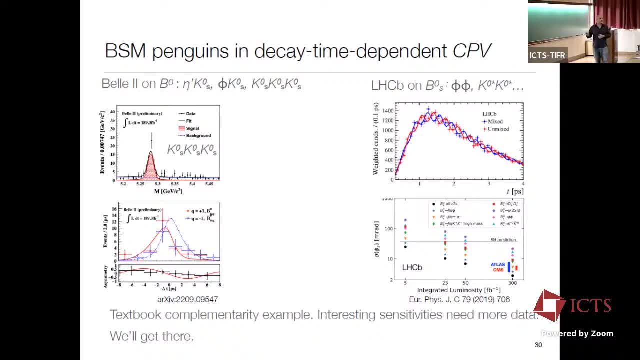 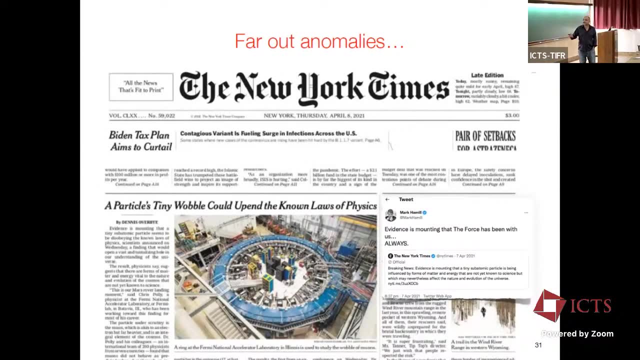 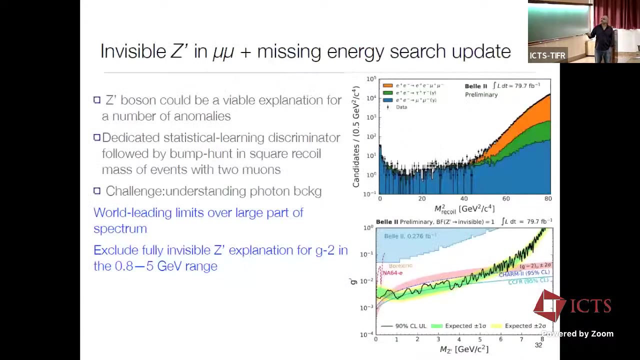 At Bell 2, you explore the b-sub-s sector on the same physics at LHCb. And finally the far-out Anomalies. we all know that the g minus 2 confirmation of the BNL result made news last year. 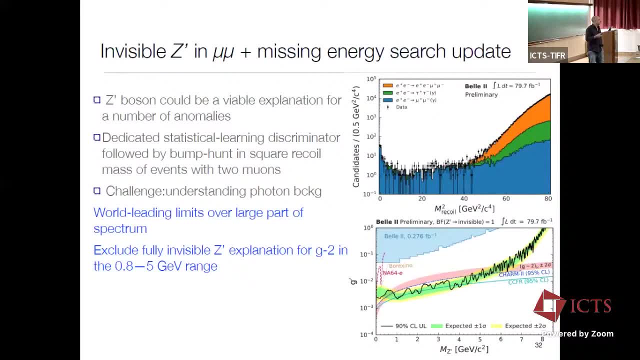 And we're trying for what we can to also contribute here. Bell 2 has a recent result on an invisible z-prime search in a final state with new mu and missing energy, which is basically a bump hunt in this spectrum of the recoil. 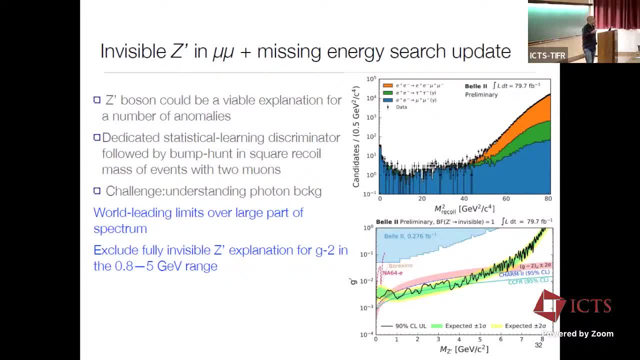 mass to the square. And this model- It's not one of the 1,000 model you can test, but it's particularly interesting because it's one of the most economic model that could explain the g minus 2 anomaly. So you see, this is the g minus 2 anomaly. 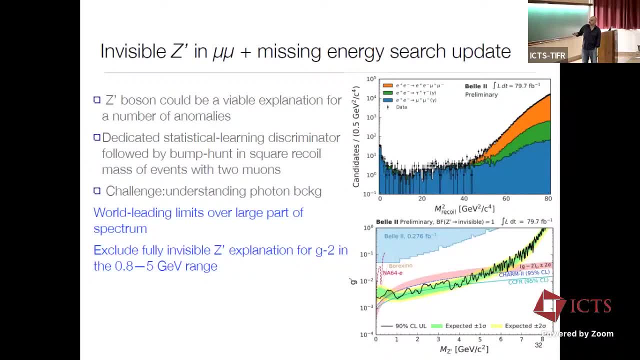 What you would expect if it was caused by a z-prime with this characteristic, And this is the exclusion limits by Bell 2, which, as you see, exclude this explanation in the range from 1 to about 5 Gv For the hypothetical z-prime mass. 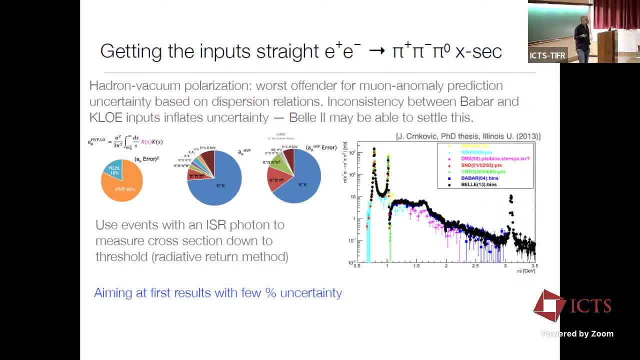 And we also try to contribute to the standard model side of this. You know that the g minus 2 standard model prediction based on dispersion relations are basically crippled by the fact that the hydrogen vacuum polarization input that comes from experiments is inconsistent between cloyer results and the bar result. 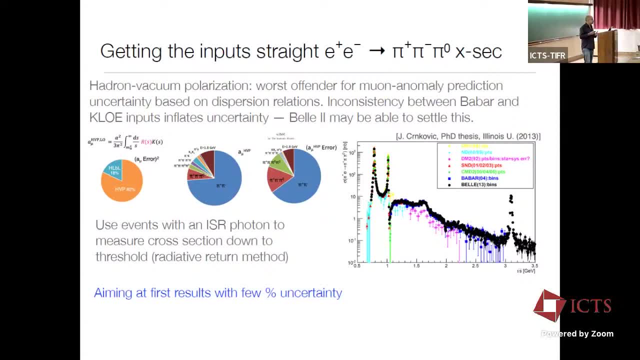 So here Bell 2 has clearly an opportunity to contribute. If we can manage to find a measurement that is very precise and very convincing, we can settle this and help improving the precision of this theoretical prediction. So we're just making the first steps in this direction. 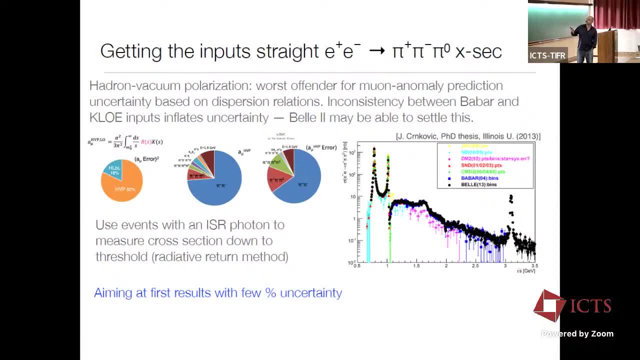 with a measurement of e plus e minus 2, pi plus pi minus pi 0,, which is not the largest contributor to this uncertainty, But it's significantly easier than the pi pi which will follow, And so we thought it was a good way of starting from there. 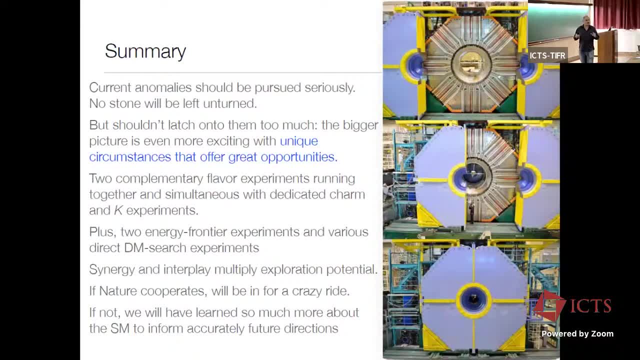 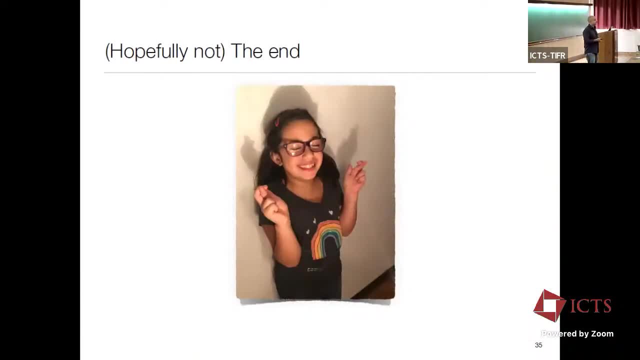 OK, Sorry, So this is my summary. I don't think I need to repeat it. I already said it many times And that's the end of my talk. I hope it's not the end of this topic, though. Thank you. 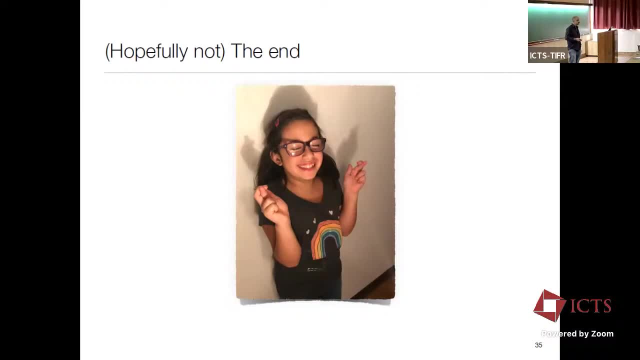 Toneli for this nice coverage of a huge topic. I see quite a few questions, A few hands raised. So let us start with the younger ones. So OK, you Not so young Hi. So from the reports of Bell 2, I see 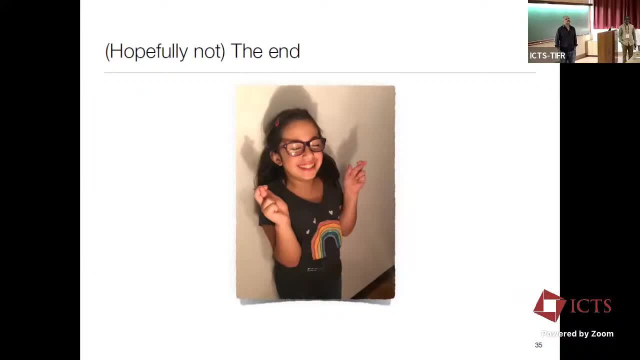 that there is some plan to measure asymmetries in tau decays like tau plus 2 pi plus k0 nu and tau minus 2 pi minus k0 nu, so on and so forth, And in many cases I see that 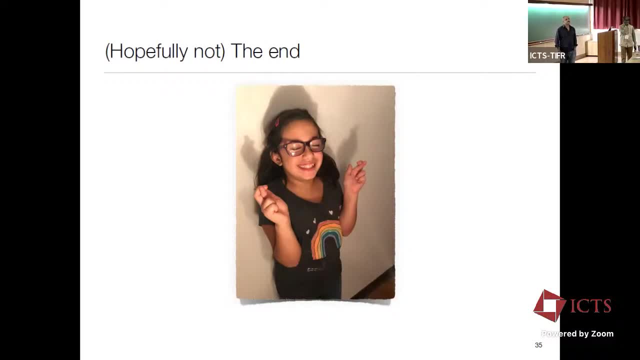 You have this tau 2 k0 and stuff channel that we expect to measure very precisely, But I never see the tau 2 k plus pi 0 channel mentioned as frequently. Is there any reason for that, Or just because of the observables? 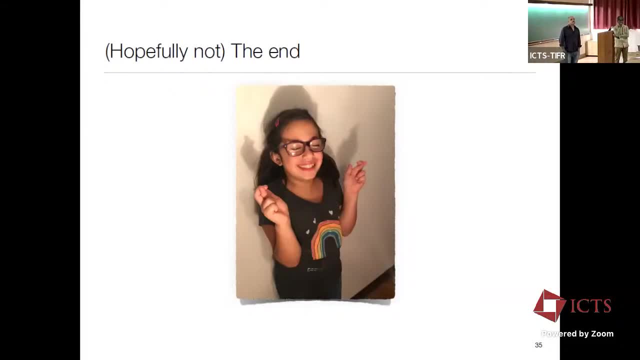 that you are more interested in, Or is there some deeper experimental thing going on? No, No deeper experimental thing going on. So is it Prioritize? We just prioritize our talk, I think, depending on the data we have and the people we have. 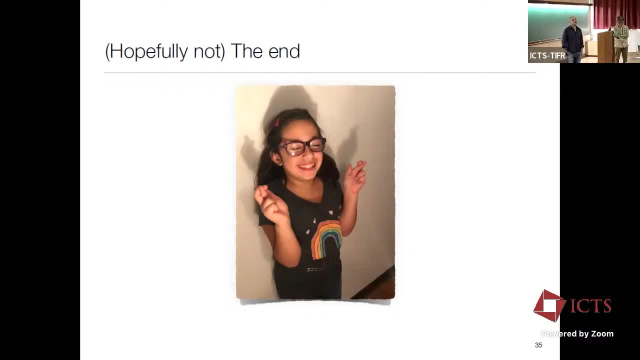 So if one like, let's say hypothetically, can give you a scenario where you can like, it might be useful to probe the tau plus, like tau 2 k plus pi 0 nu channel, and then take the ratio with the tau plus 2 k0 pi plus channel. 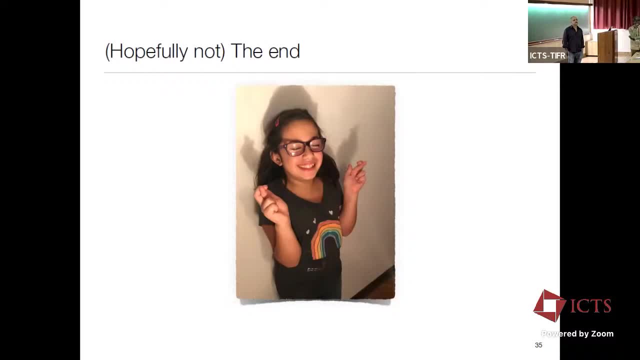 like. if it can be experimentally, like sorry, theoretically motivated, then there's no reason why you cannot look at that ratio at a very high precision. OK, OK, thank you. OK, Yeah, thank you, Yeah, so I'm here. 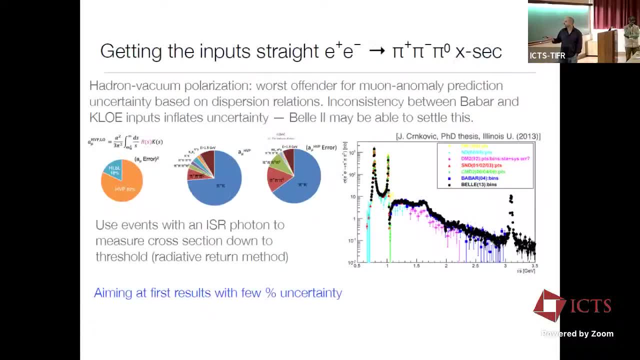 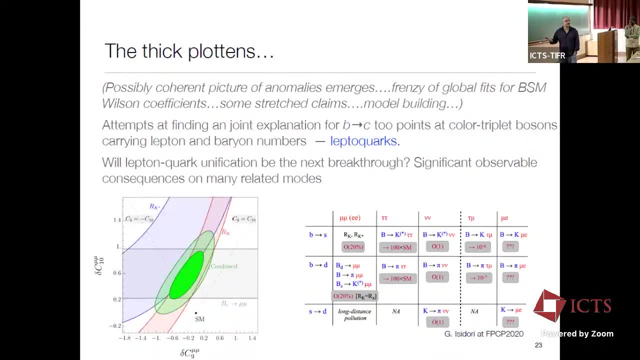 So I have a question on slide 23, where you showed that formula for lepton flavor universality and how you probed that: Yeah, yeah, this one, this one, yeah, Oh, this this. No, no, no, the lepton flavor universality. 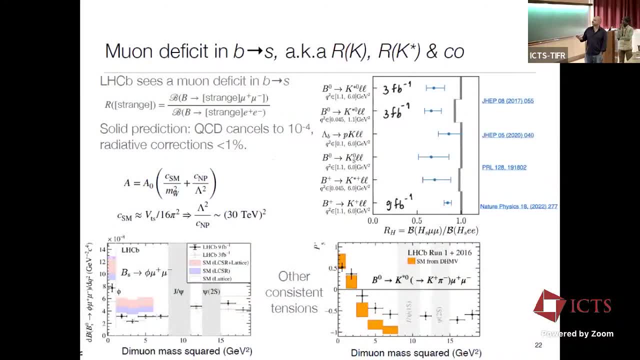 I guess it was the slide we just passed by This. Yeah, so in this formula, when r strange going to the, basically the ratio between the branching fractions of mu plus and e plus, e minus. So what prevents you from computing this in the tau sector? 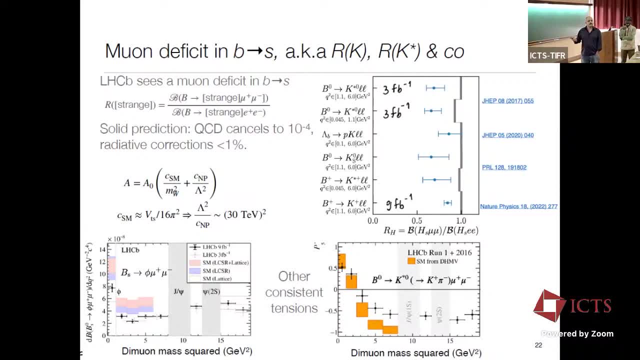 as well say tau to mu or e to tau. Like what's wrong with that Tau reconstruction, say in the adrenic channel? Yeah, yeah, there are tests of lepton flavor universality. You mean tau decays. 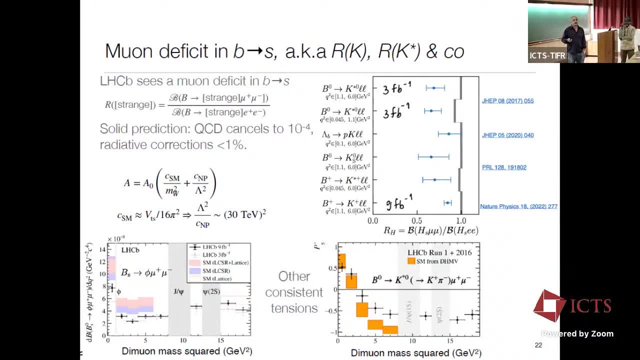 Exactly tau decays There are. there are. we are pursuing that And people have predictions for that, Like combining the results for the two channels. That's what that was my question Like. are you working on that as well? 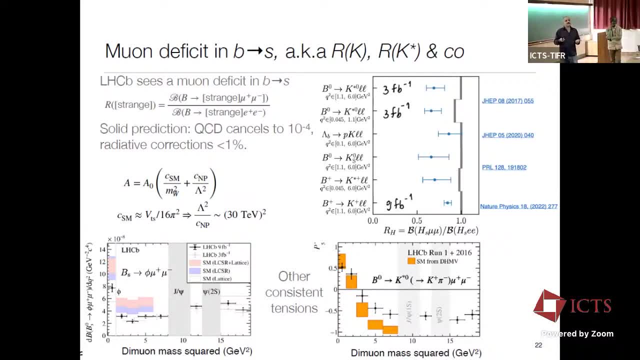 Yeah, yeah, we're working on everything. The difficulty is getting the result out, Although this is not the main topic of your talk about the g minus 2.. As you said, there is an inflation in the error because of the inconsistency between and that you could settle that. 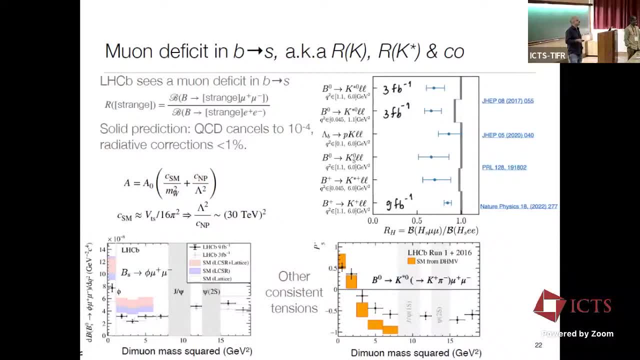 And yet, And yet, even with that inflated error, there's no way one can account for the discrepancy between the experiment and the theory today. And this, of course, look at the lattice, which is somewhere in between. Yet I think the lattice error is probably underestimated.